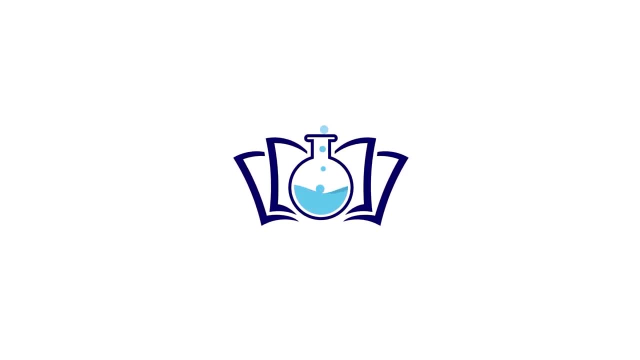 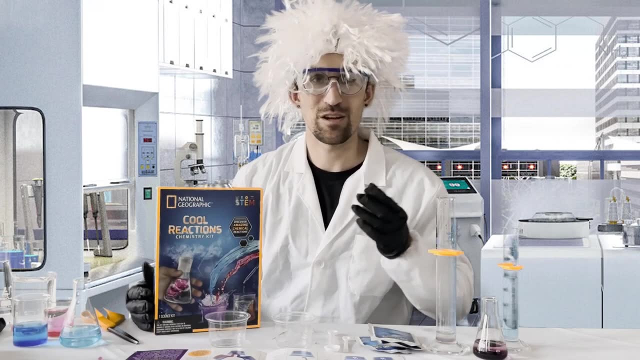 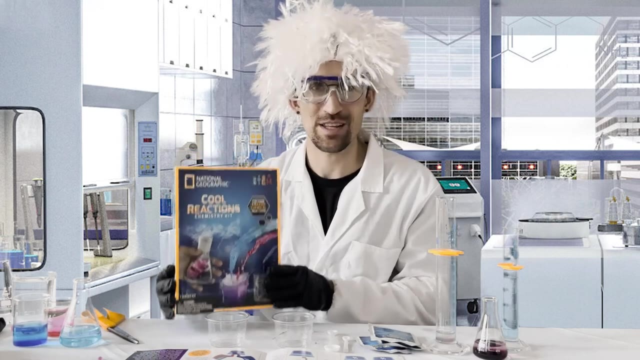 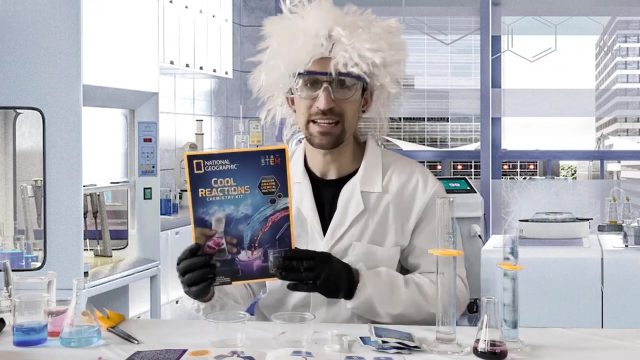 Scientists. hello and welcome back to the laboratory. Today we're going to do an exciting experiment from the National Geographic Cool Reactions Chemistry Kit- link you can find in the description- to make a big fizzy eruption. Now, everything we need today is included in this kit. 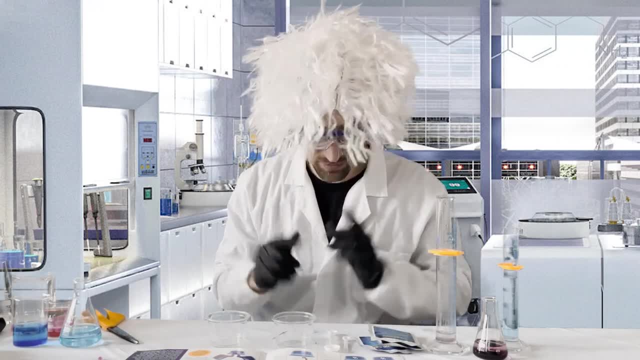 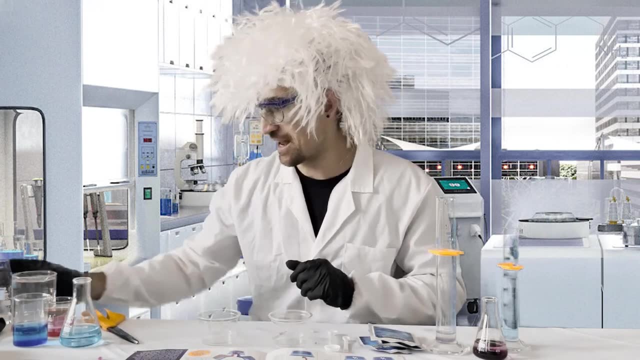 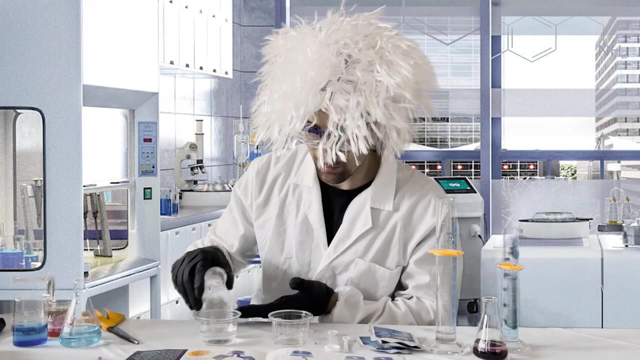 We're just going to bring our own room temperature water. So to get started here, I have in front of me two of our different little measuring cups. I have my room temperature water and I'm going to start by filling both of these up about halfway with water. There's one, there is another, The 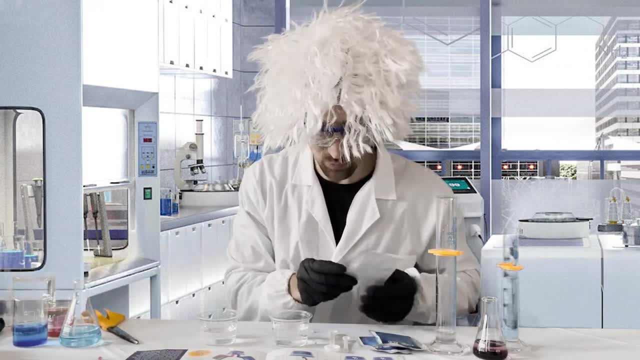 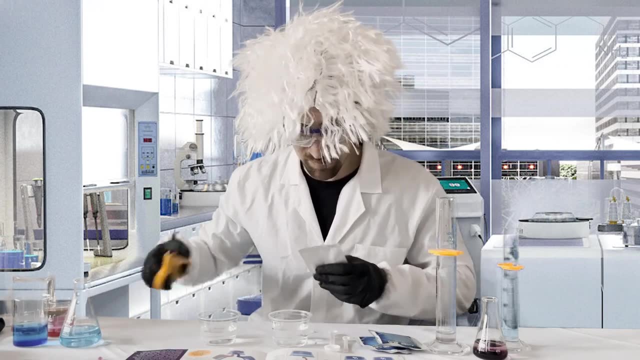 next step I'm going to do is I'm going to go ahead and use this red cabbage powder and I'm going to fill them up with water. I'm going to fill them up with water and I'm going to fill them up with one small scoop. Now, keep in mind, your kit is going to contain two different size scoopers. You 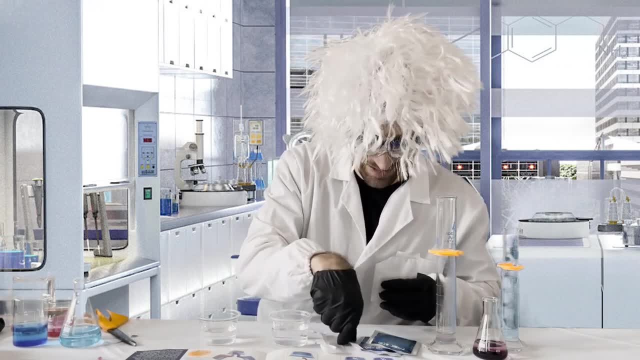 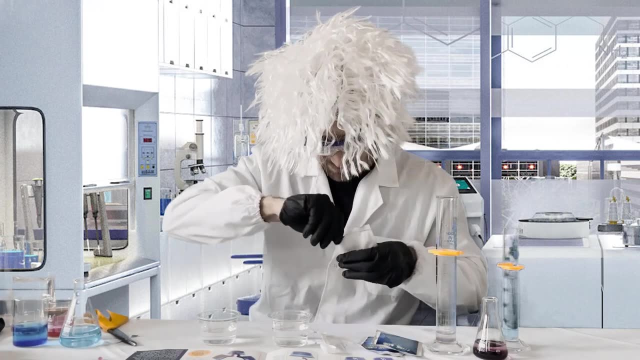 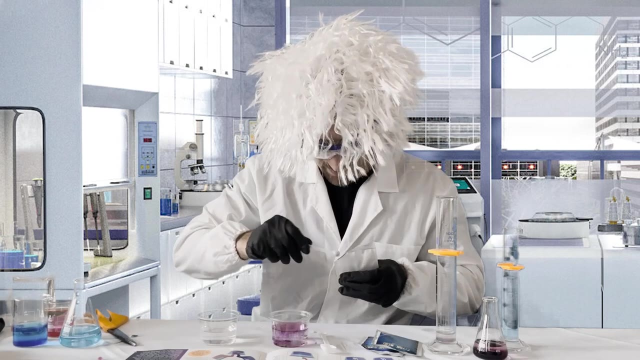 have your spoon with two ends and then you have your small tiny scooper. We're going to use our tiny scooper right now, So I'm going to go ahead and I'm going to pull one little scoop and it goes and you can see it's immediately having an effect here. It's going and it's coloring that water. 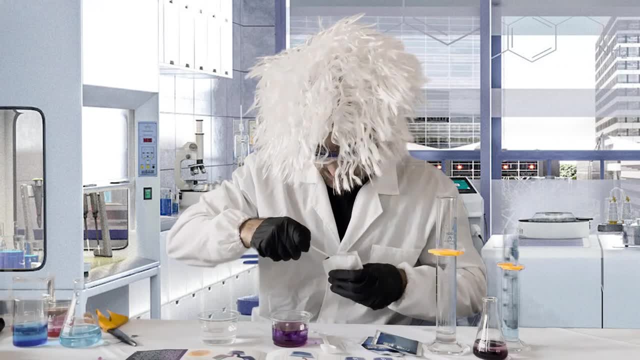 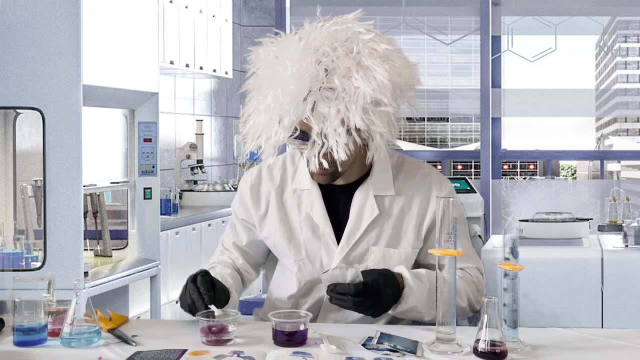 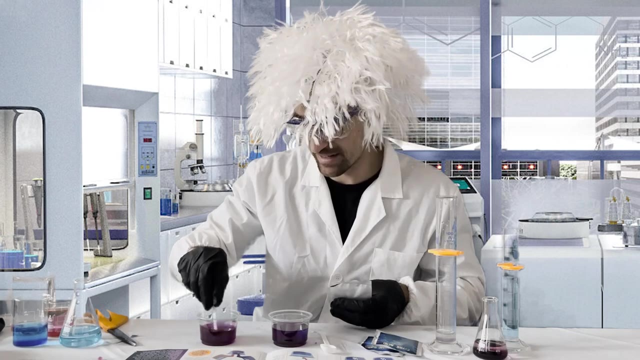 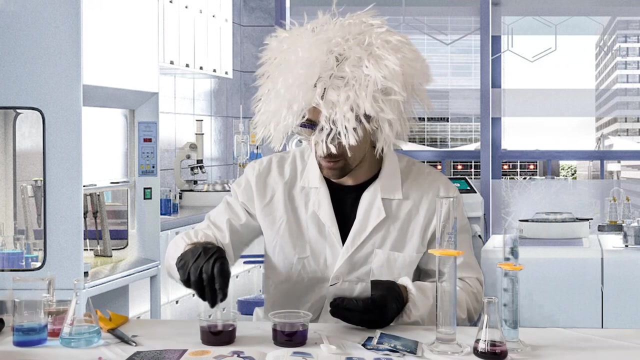 I'm going to take another small scoop. put that in there again Now. for those of you that may not have seen the other experiments, keep in mind that red cabbage powder does act as an indicator, So it changes color based on the acidity of the solution it's in. Something could be more acidic or more basic. We're going to. 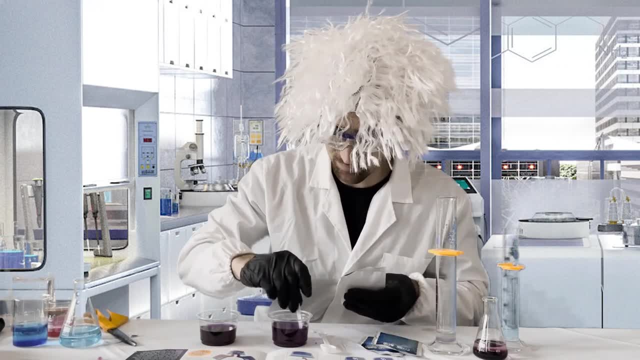 just go ahead and mix it, just to make sure that that powder is going to be in there. So I'm going to pour more right now. I have two cups in here that I just didn't add, theら. We're going to mix all these very nice a little bit, So we're going to have about 60 steht right now. So it is not. 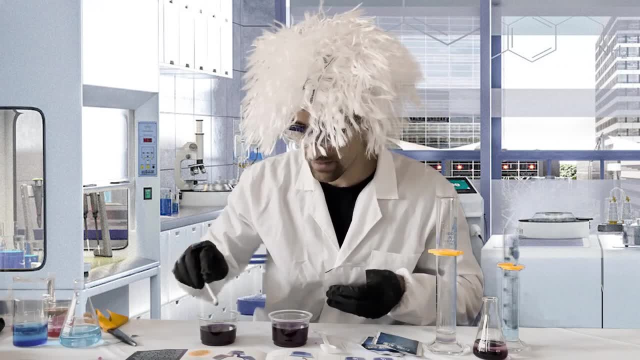 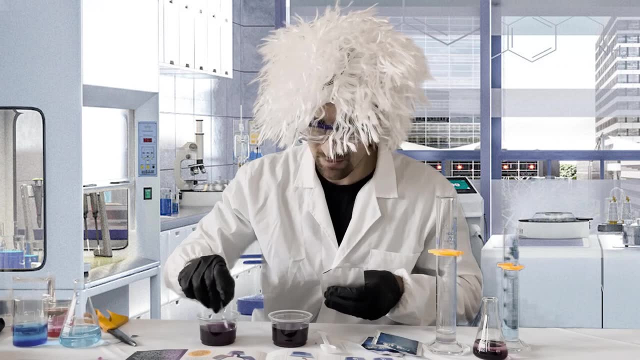 complicated to mix these in, and our water is boiling. We're adding the red cabbage powder. You can see, as I added, the rye cabbage powder is fully dissolved and we've created this solution of red cabbage powder and just room temperature water. Now what we're going to do next is we're 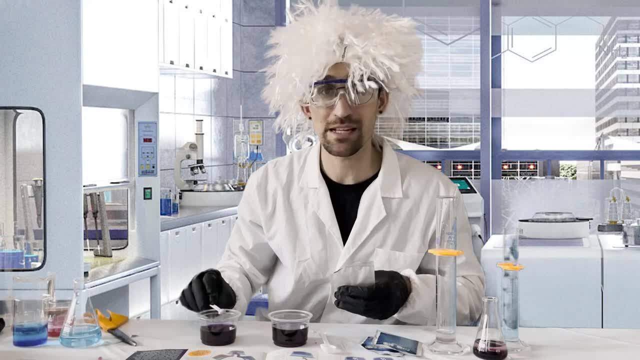 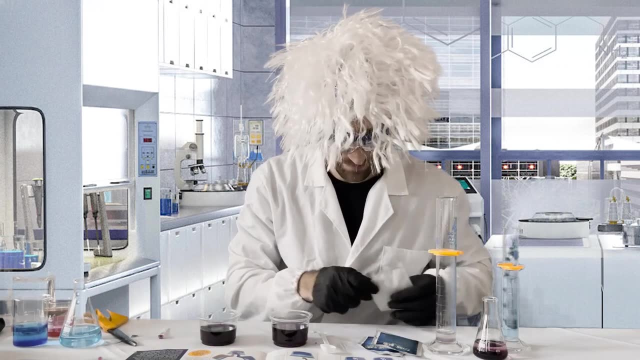 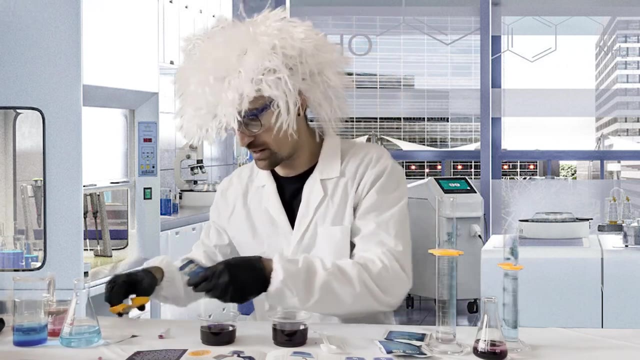 going to alter the acidity of these liquids- iOSstroma basic type of a material, And so that mixing is done, I'm now going to come to my baking soda, also known as sodium bicarbonate. I'm going to go ahead and open it up. We're going to use the 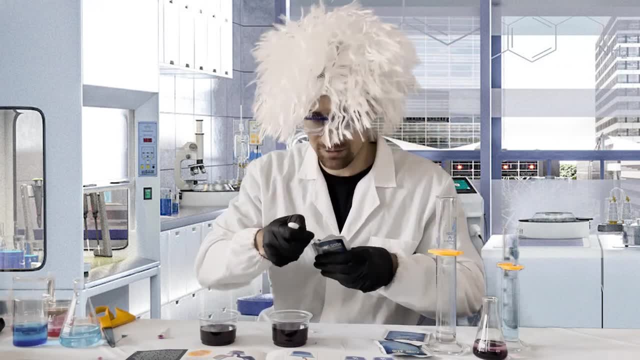 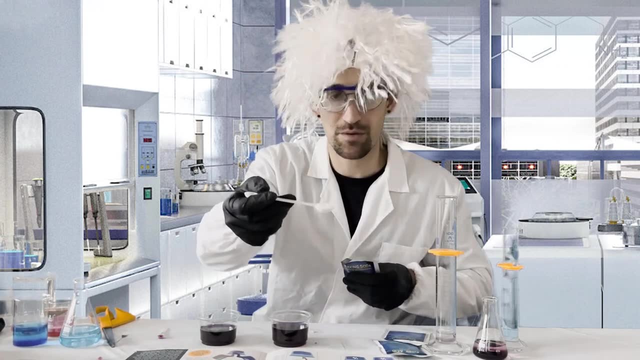 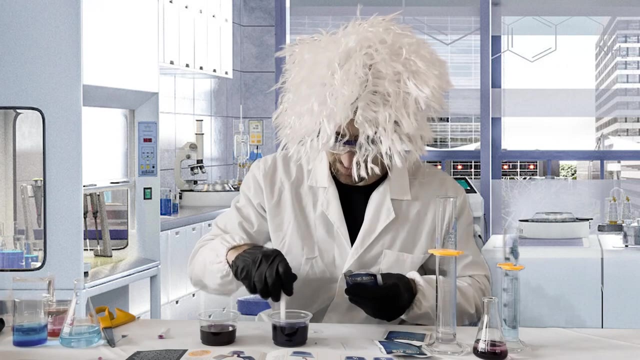 big scoop this time. So we're switching to our two-sided cup, We're using the big scoop and I've got one full of baking soda here, big scoop, and it is going to one side And I'm going to go ahead and stir this And I can immediately see the water is turning a dark, dark blue. 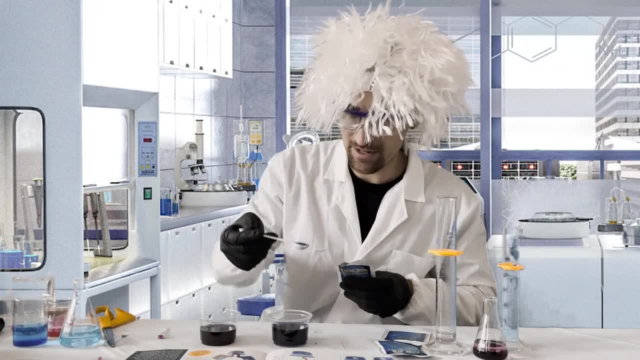 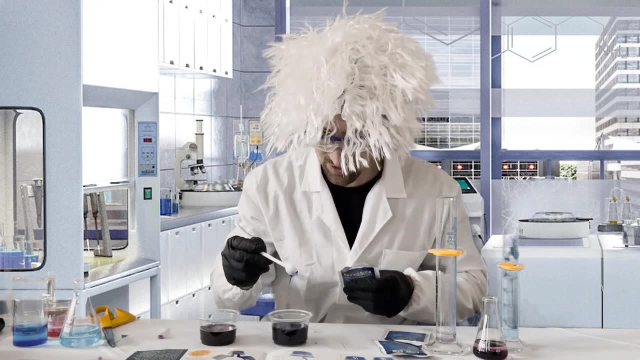 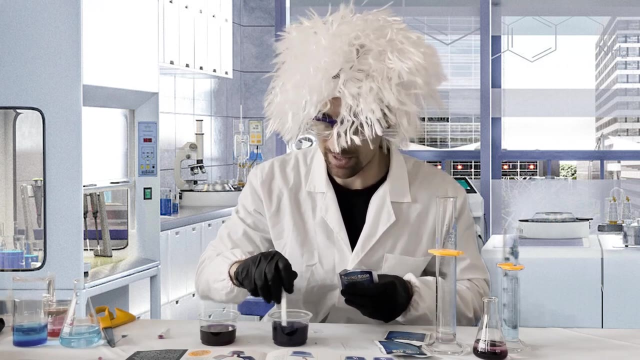 And also when you lift it out with your kind of spoon. here you can also validate that it has turned a dark blue And keep in mind that's because that cabbage liquid is. that indicates that we have a very, very basic solution on one end. Now the next thing we're going to do: 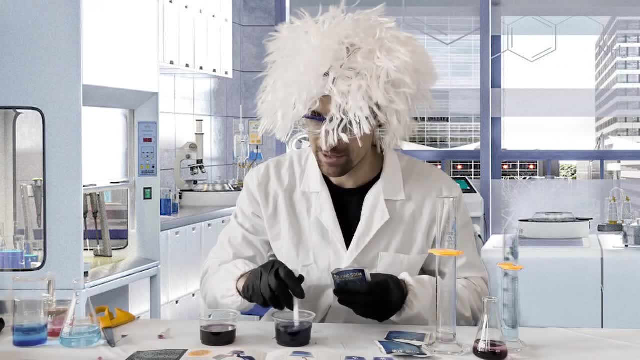 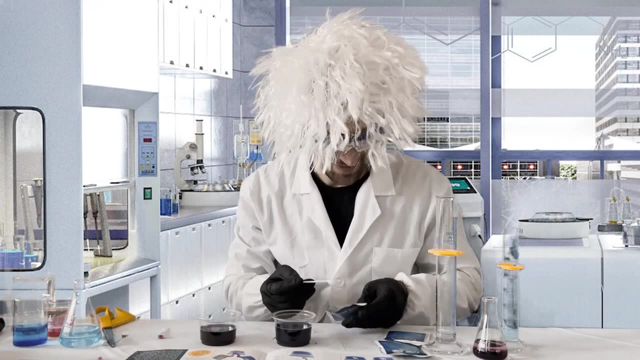 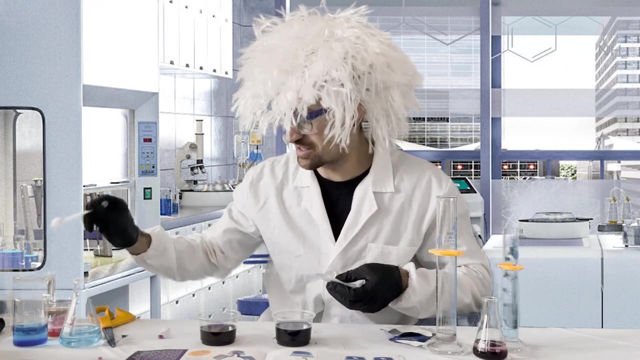 is, we're going to add one big scoop of citric acid to the other solution. Now that should turn it more red, because red indicates acidity with the cabbage powder, And so you can wash off that spoon, just not to cross-contaminate prior to dipping it into the citric acid. 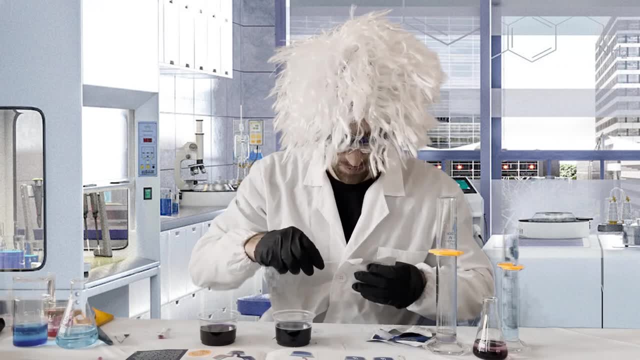 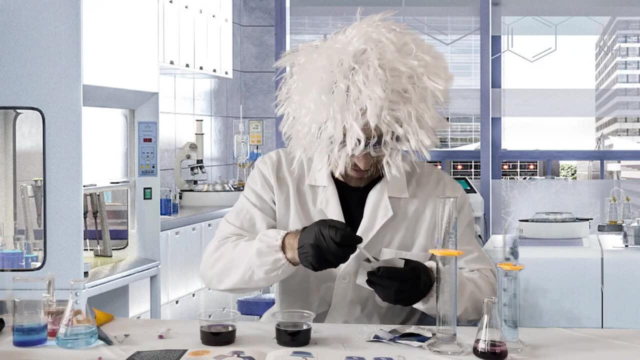 Go ahead and be careful as you open these items. You want to do it better than I do. You don't want to be messy, You want to be very careful here. So definitely, as you're doing these experiments, do it over a material that won't get stained or damaged, And so I'm just going to pour. 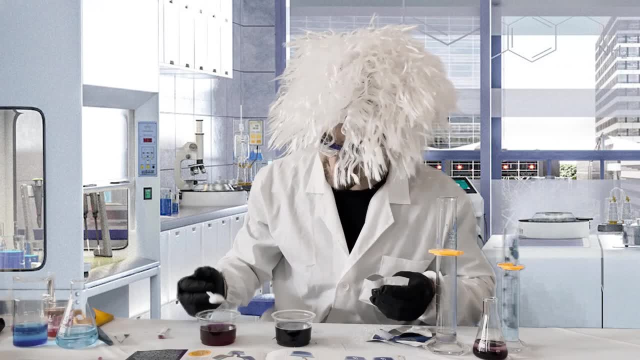 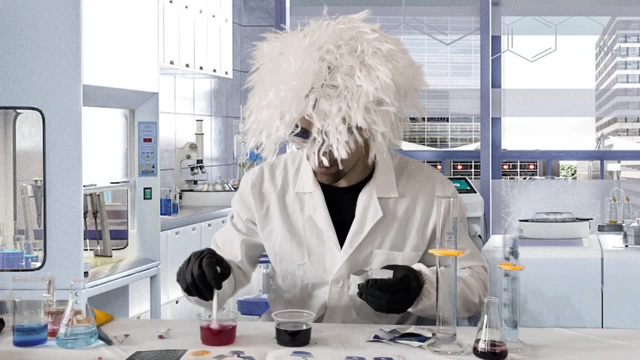 that citric acid in there, And I can immediately see it is becoming a very, very deep red there And so a lot of red. Wow, Very, very different color here, This red, because it's a very, very deep red, And so I'm going to pour that citric acid in there. 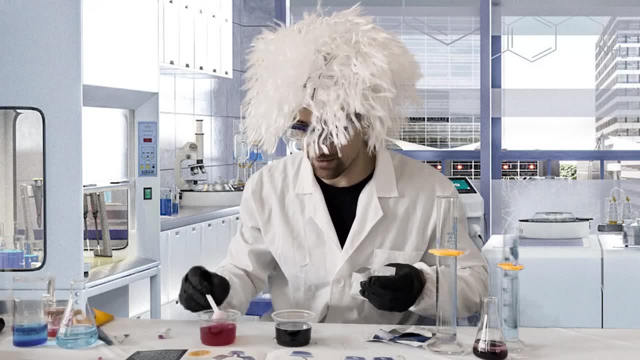 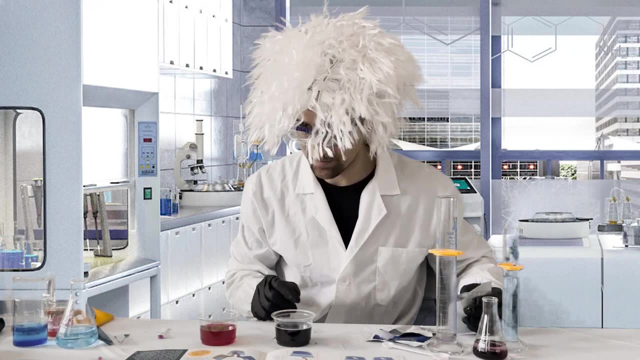 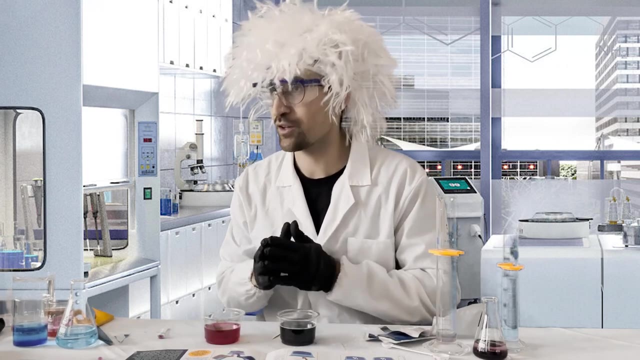 It's acidic, It's reacting to the cabbage powder, which is our pH indicator. Then our basic solution here based with that baking powder. So we have acidic solution and a basic solution here. What we're going to do is we're going to grab.